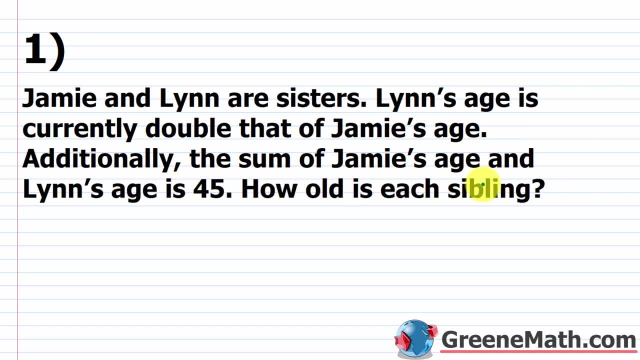 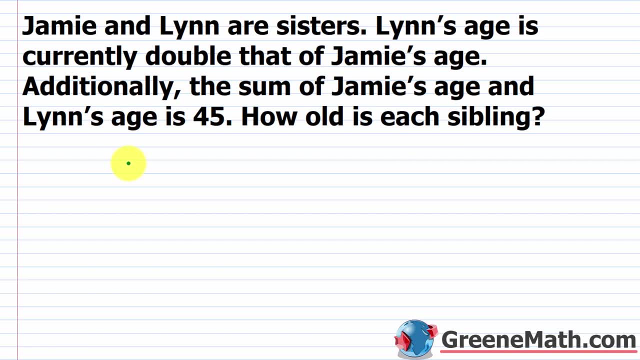 age is 45.. How old is each sibling? So the end result here is: we want to know how old is Jamie and then how old is Lynn. Now we can let x be equal to the age of one of them. It does not matter which one you pick, You can model it either way. So I'm just going to let x be equal to the. 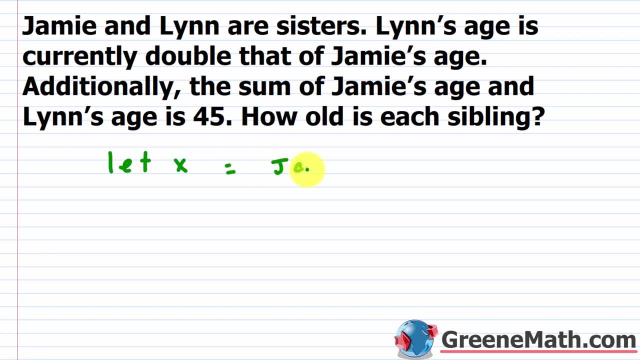 age of Jamie. So let's just put: this is equal to Jamie, So Jamie, so her age, Okay. so then how are we going to model Lynn's age? Well, it tells us here that Lynn's age is currently double that of 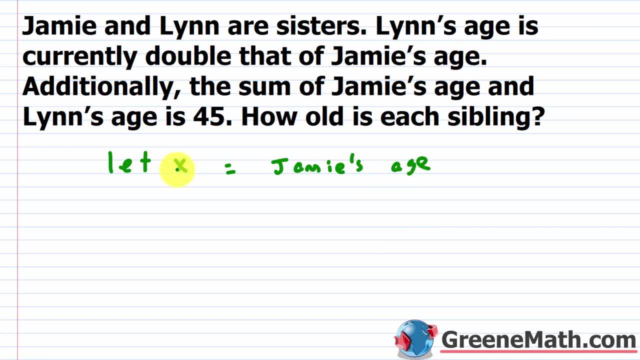 Jamie's age. So if Jamie's age is x, why need to double that? So that's two times x to model Lynn's age. So what I'm going to do is I'm going to put then, and I'm just going to go to: x is equal to, and then I'm 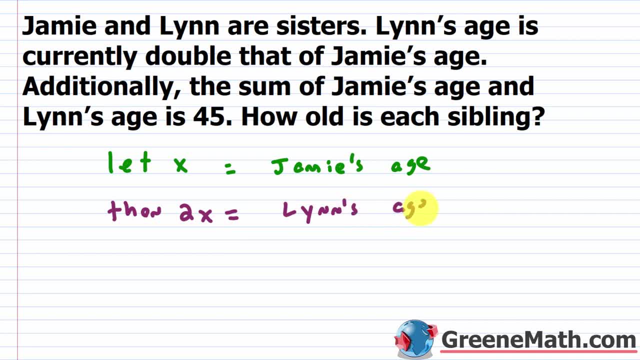 going to put Lynn's, so Lynn's age like this: Okay, so we've modeled that, And now we want to move on to creating an equation. So how do we do that? Well, it tells us additionally the sum of so the sum of Jamie's age and Lynn's age is 45.. 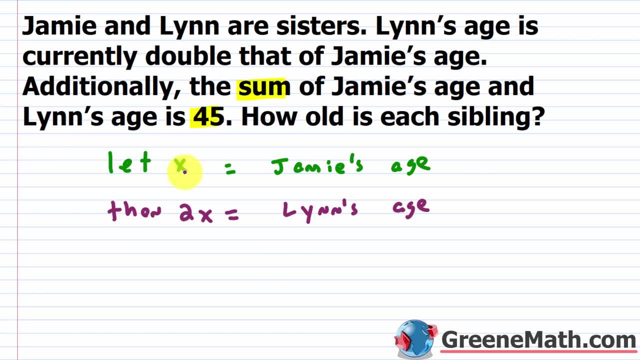 So all I really have to do for this problem is take x, which is Jamie's age, and add it to 2x, which is Lynn's age, And I know the sum here is going to be 45. Because, again, that's given to me. 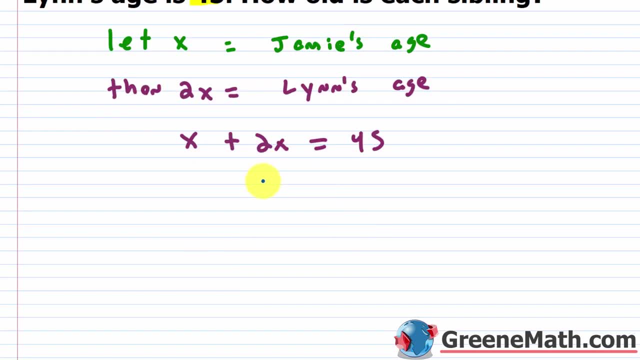 in the problem. So this is a really easy equation to solve. x plus 2x is 3x, And this equals 45. Let's divide both sides of the equation by three, And so let's cancel this with this, And we'll say: 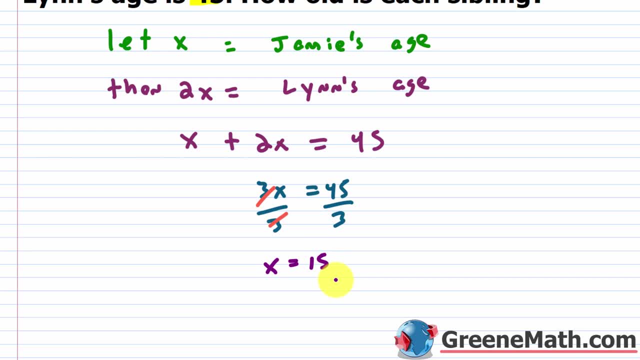 that x is equal to 15.. Now again with a word problem, you have to go back and do some additional work to answer your problem. x was Jamie's age, So we know in this case this is going to be 15.. 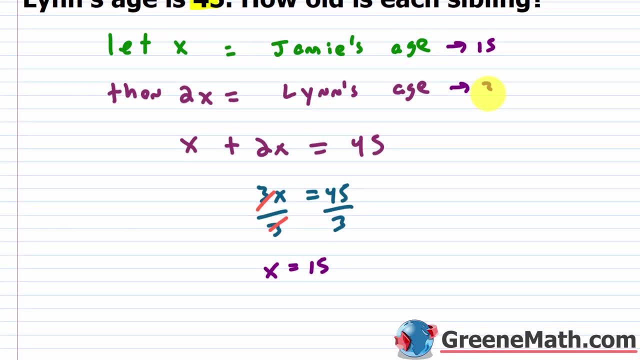 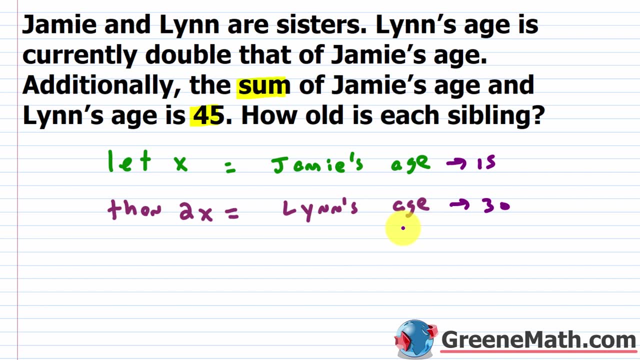 So then 2x was Lynn's age. In this case that's going to be 30. So at this point you could make a nice little sentence and say that Jamie is 15 years old and Lynn is 30 years old In the 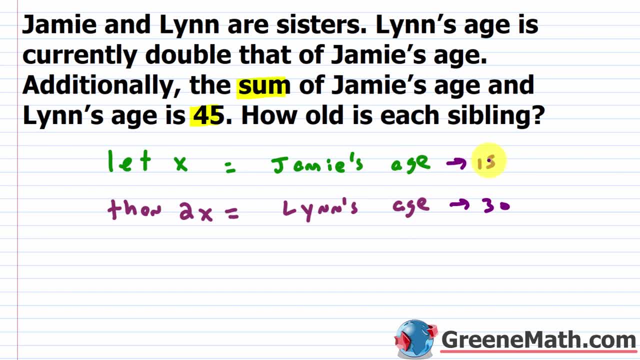 interest of time, I'm just going to leave my answer like this, just saying that Jamie is 15 and Lynn is 30. And if you want to go back through the problem and check things, it says that Lynn's age is currently double that of Jamie's age. Well, Lynn is 30 and Jamie is 15.. 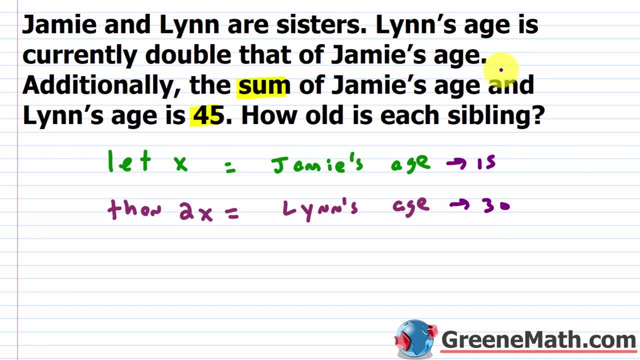 So that checks out. And then here, additionally, the sum of Jamie's age and Lynn's age is 45. Well, 15 plus 30 is 45. So our answer here is correct. Again, Jamie is 15 years old and Lynn. 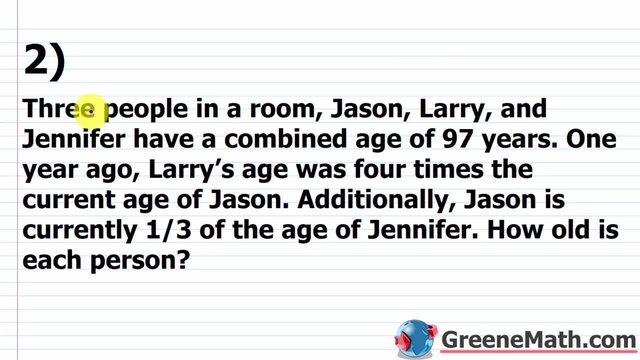 is 30 years old. All right, let's look at problem number two. So now we're told that three people in a room- we have Jason, Larry and Jennifer- have a combined age of 97 years. Let me actually highlight that that's going to be important. So then it says: one year ago, Larry's age was four times the 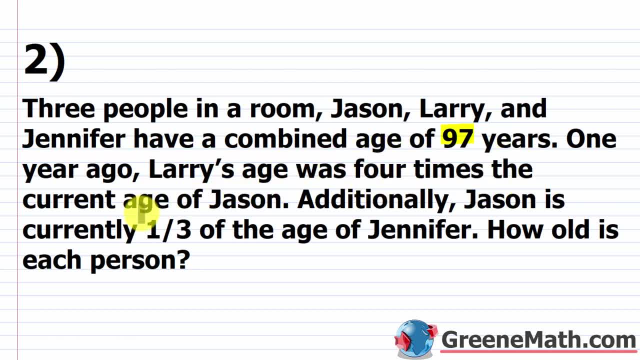 current age of Jason, And then we're told that three people in a room we have Jason, Larry and Jennifer. Additionally, Jason is currently one third the age of Jennifer. How old is each person? So how old is Jason, How old is Larry And how old is Jennifer? So the first thing is: 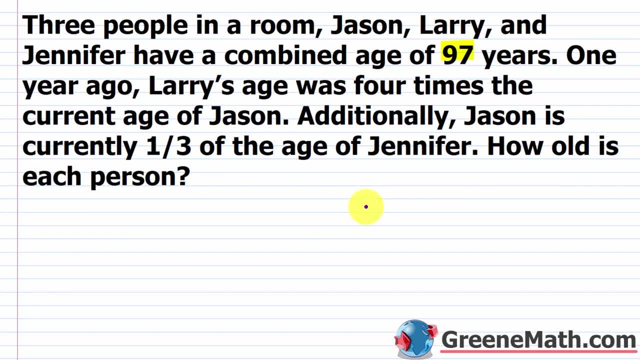 we're going to let a variable like x be equal to the current age for one of these guys, And what I would do is always look for the person that's involved in each comparison. So, first and foremost, it says that one year ago, Larry's age was four times the current age of Jason, And then you see. 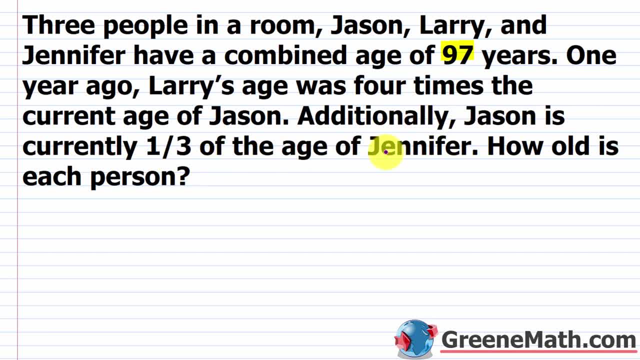 Jason again. Additionally, Jason is currently one third of the age of Jennifer. You don't have to do that, So let's take the person that's involved in both comparisons and start off with that. So I'll say: let x be equal to. this would be the current age of Jason. So let's put Jason's, So Jason's age, Okay. so then how are we? 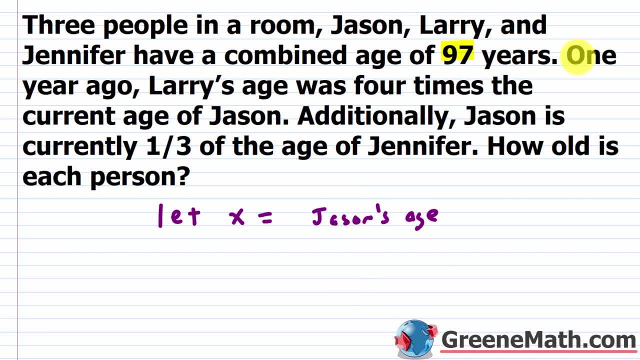 going to figure out what is the age of Larry. Well, it says one year ago, Larry's age was four times the current age of Jason. Okay, so let's start with four times the current age of Jason. So I'm going to put then again we. 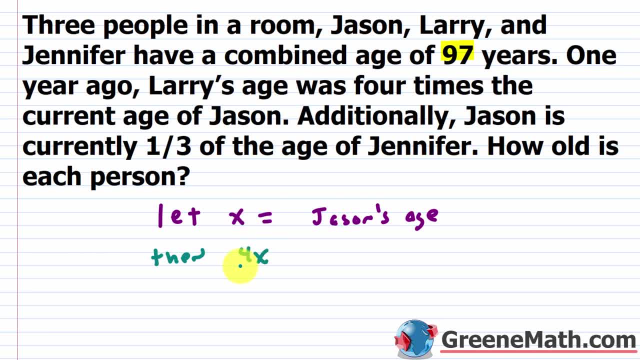 have four times the current age of Jason is x. So I'm just going to go for x now. is for x representing Larry's current age? No, what does it represent? Well, again, it says Larry's age was four times the current age of Jason. 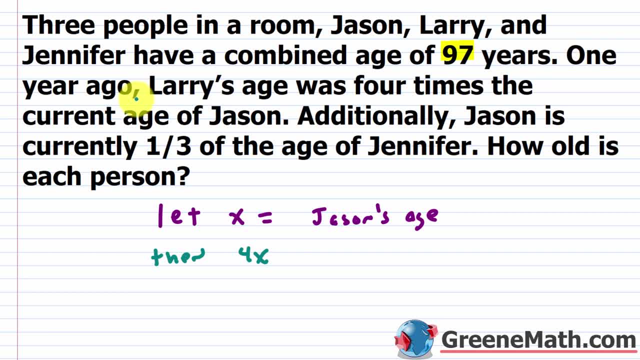 And this was one year ago. So what I have to do to get to the current time period, since this was a year ago, I have to add one, So plus one here, And then this is going to be Larry's current age. So this is Larry's age. Okay, Now for the last. person it says additionally, Jason is currently one third of the age of Jason. So let's say that's four times the current age of this person. So let's say I start misplacing this player. wow, you thought you would get this right. And so to add the old kid. 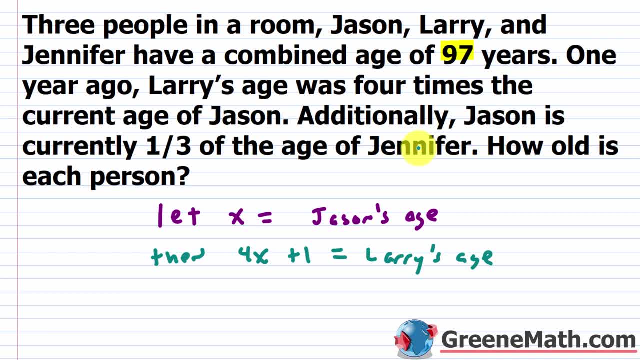 you close the next one back and this is how to add the new program. But what's good about three is its age actually is currently one third of the age of Jennifer. So if Jason is a third of the age of Jennifer, that means Jennifer is three times as old as Jason. So basically what I can do, I'll say 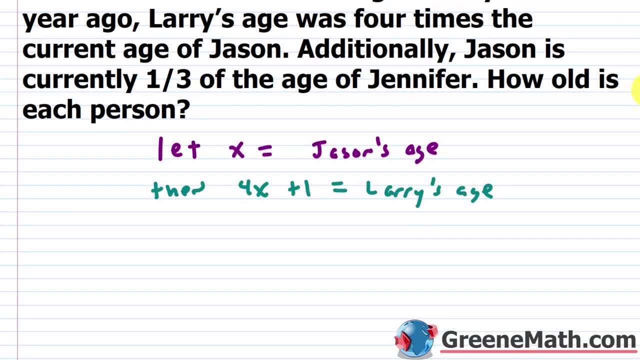 then we'll go three times. x is going to be equal to. this will be Jennifer's age. Okay, so now that we have this modeled, again going back up, we know that they have a combined age of 97 years. again, this is told to us in the problem. So basically, guess where we're. 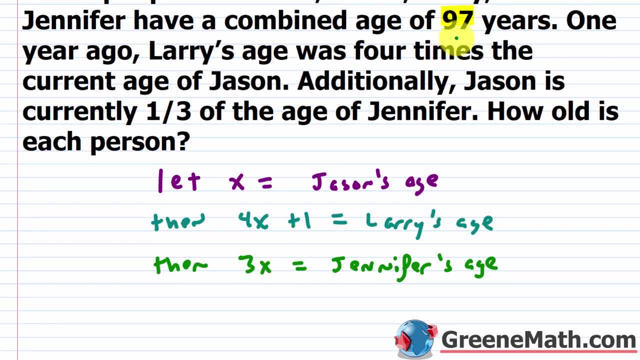 going. Okay, it's in this old age, So Y eight. turning on the use case data, we use this word that I just touched up And it says 97 years. Again, this is told to us in the problem. So all we really need to do is set up an equation. 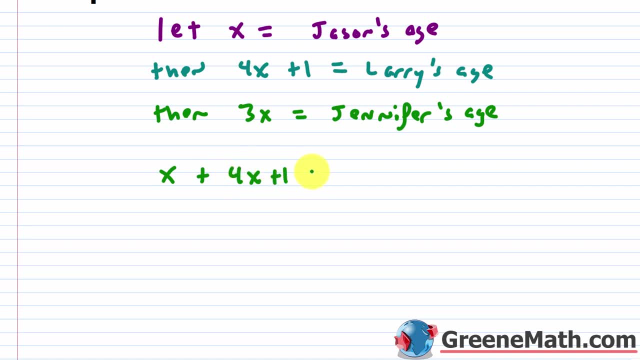 and say x plus this, 4x plus 1 plus 3x is equal to 97. So again Jason's age plus Larry's age plus Jennifer's age, that should give me 97. So going through here, x plus 4x is 5x, then plus. 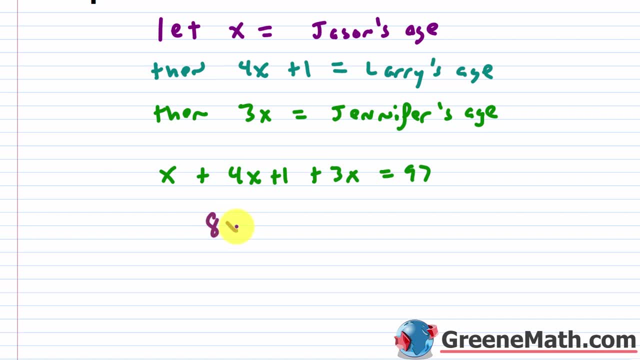 3x is going to be 8x, So this is going to be 8x plus, and then you just have the 1, this equals 97. Then we're going to subtract 1 away from each side of the equation. This will cancel You're. 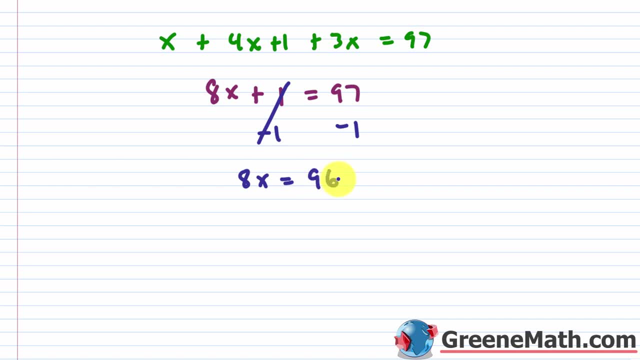 going to have: 8x is equal to 97 minus 1 is 96.. And then, to finish this up, let's divide both sides of the equation by 8, and let's cancel this with this, And so what I'll have here is that x is. 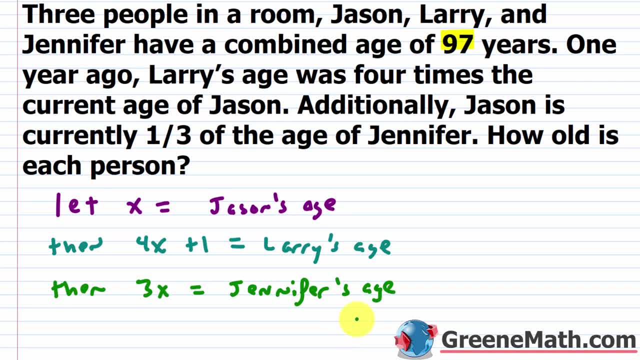 equal to 96 divided by 8 is 12.. Okay, so, coming back up here again, x was 12.. So this is Jason's age, So he's going to be 12 years old. We go 4 times 12,, that's 48, plus 1 is 49. So that's going. 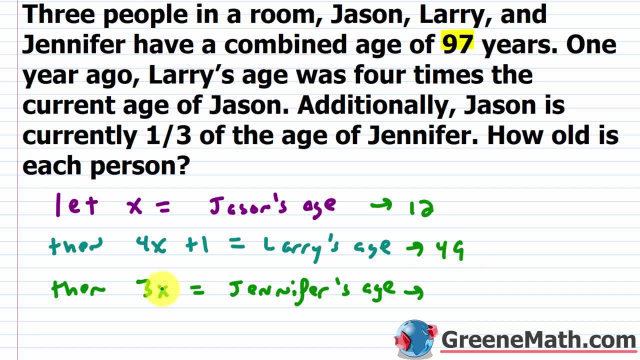 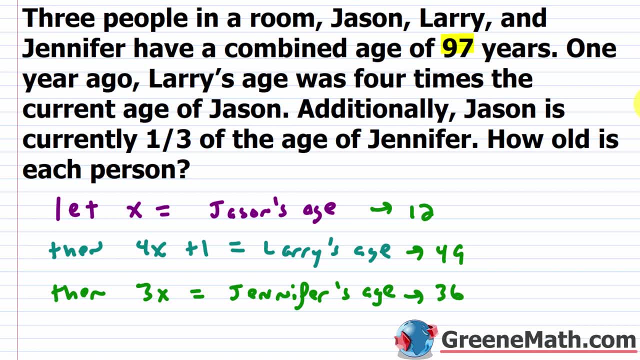 to be Larry's age, And then again for Jennifer. she's 3 times 12, or 36.. Okay, reading back through the problem to see if these answers are correct, Again, they have a combined age of 97 years, So 12 plus 49. 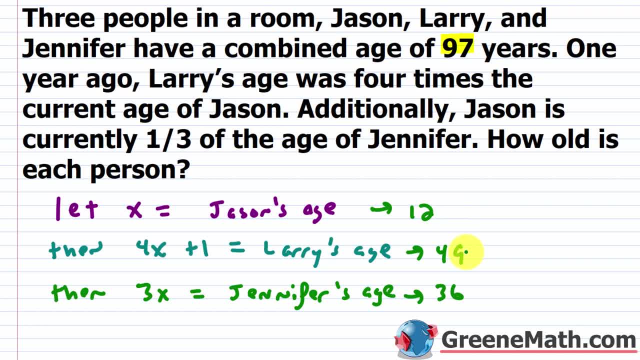 is 61, then plus 36 does give me 97. So that part checks out. And then it says one year ago Larry's age was four times the current age of Jason. So a year ago Larry would have been 48,. 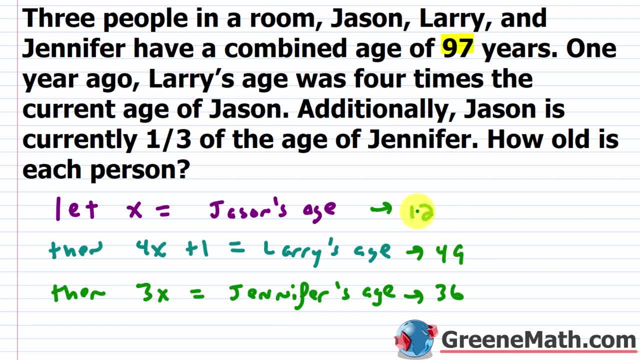 and 48 is four times the current age of Jason, which is 12.. So that checks out. Then it says, additionally, Jason is currently one third of the age of Jennifer. Well, Jason is 12, and Jennifer is 36.. 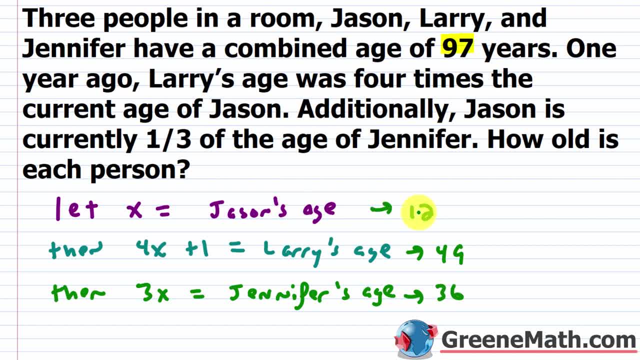 So that checks out as well. So again, we have our answer here. If you want to make a nice little sentence with it, you can. I'm just going to leave it like this. We'll say: Jason's age is 12.. 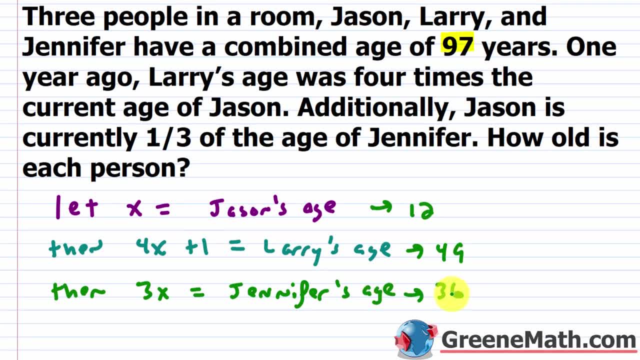 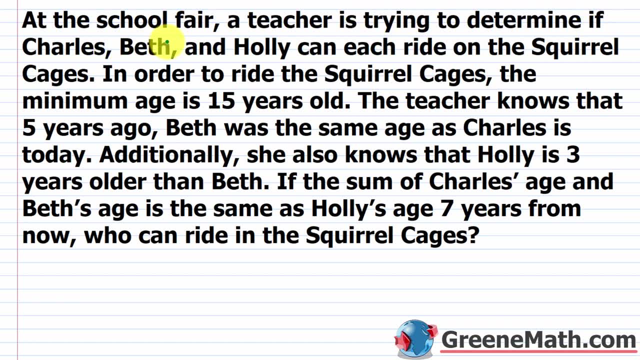 And then Larry's age is 49. And then Jennifer's age is going to be 36.. Okay, let's look at problem number three. So we have, at the school fair, a teacher is trying to determine if Charles, Beth and Holly can each ride on these squirrel cages. 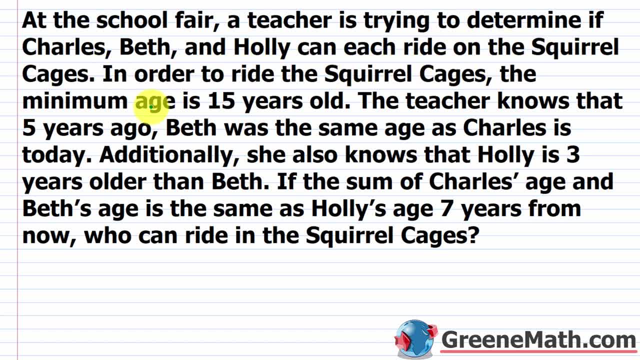 So, in order to ride the squirrel cages, the minimum age is 15 years old. The teacher knows that five years ago, Beth was the same age as Charles is today. Additionally, she also knows that Holly is three years older than Beth If the sum of Charles's age and Beth's age is the same as. 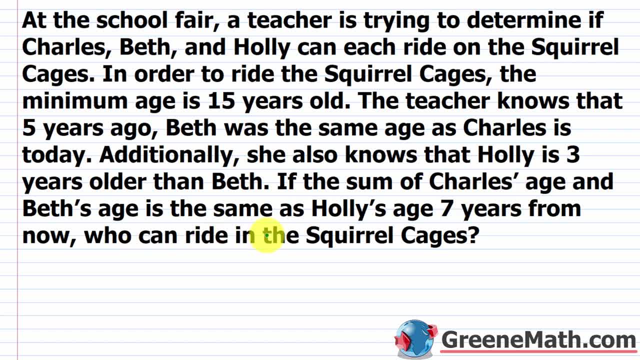 Holly's age, seven years from now, who can ride in the squirrel cages? Okay, so let's think about this and just go step by step. Again, we need to know the age of each person and then we need to figure out: is this person going to be 15 years or older so that they can ride on the squirrel cages? 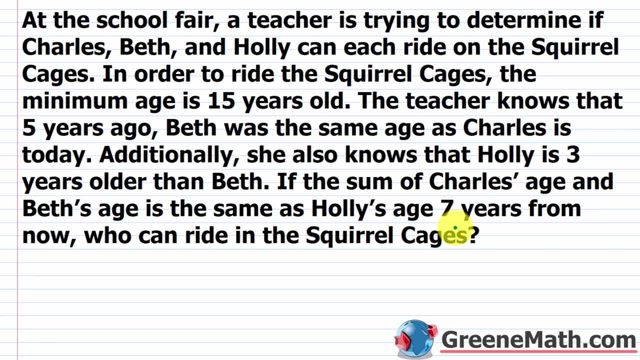 So again, it's usually easiest to think about the person that's involved in each comparison. So here you have Beth and Charles, and then here you have Holly and Beth. So Beth is involved in each comparison. So I'm going to start out by saying I'm going to let X 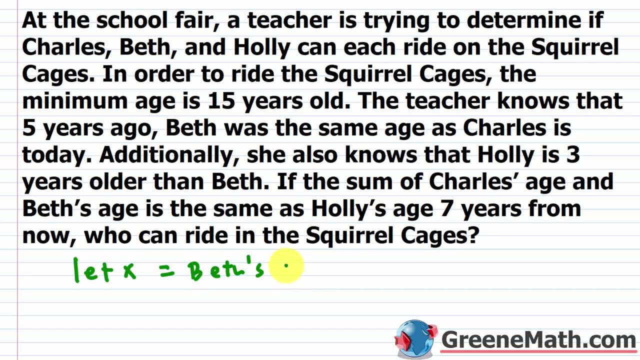 be equal to Beth's age. So this is Beth's age, like this. And then, when I think about this sentence here, the teacher knows that five years ago Beth was the same age as Charles Charles is today. so that just means that Beth is going to be five years older than Charles. 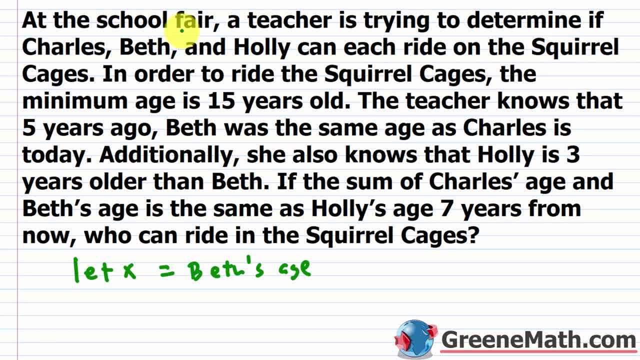 or you could say that Charles is five years younger than Beth. so basically, I can just say that then all we have to do is say: x minus five is going to be equal to Charles's age. so this is Charles's age, and then let's read the other one. so, additionally, she also knows that 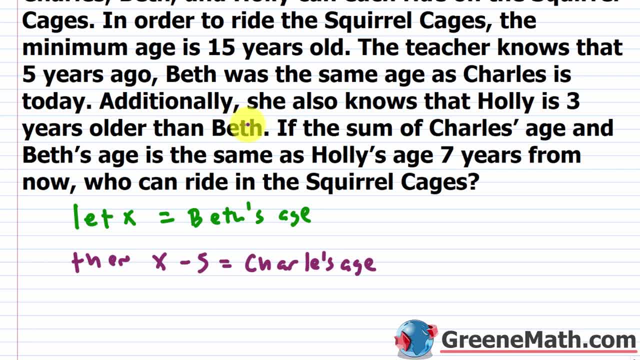 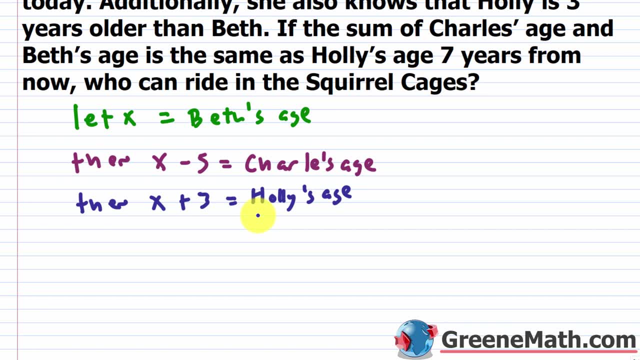 Holly is three years older than Beth. so basically take Beth's age, which is x, and just add three to that. so we'll say then: now we can say x plus three is going to be Holly's age, so this is Holly's age. so now that we have these guys modeled here, we're told if the sum of Charles's age and Beth's 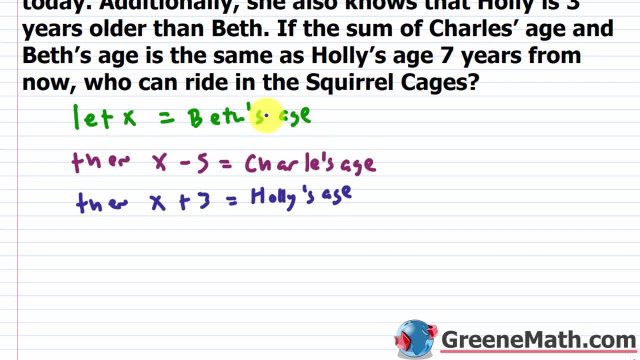 age. so the sum of those two- here's Charles's age, here's Beth's age. so basically it's x plus your x minus five. we're summing those two together, we're saying is the same as. so that means equals. we have Holly's age seven years from now. 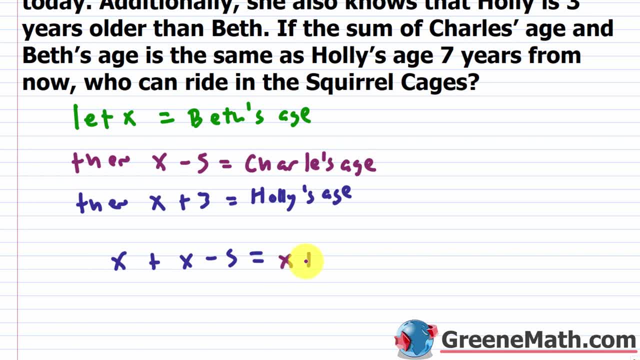 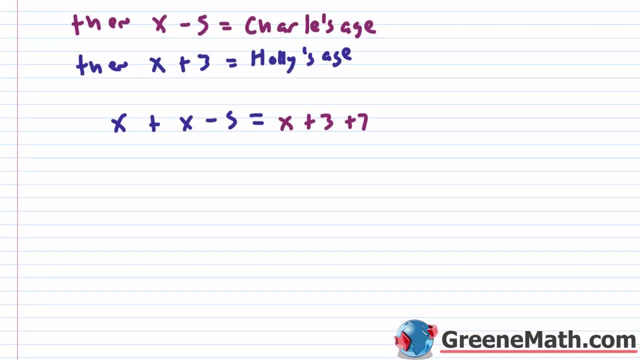 so here's Holly's age. right now it's currently x plus three, and in seven years I would just add seven to that. so plus seven, okay. so let's go through and see what this gives us here, and I'm going to basically say: x plus x is two, x, then minus five is equal to: we'll have over here on. 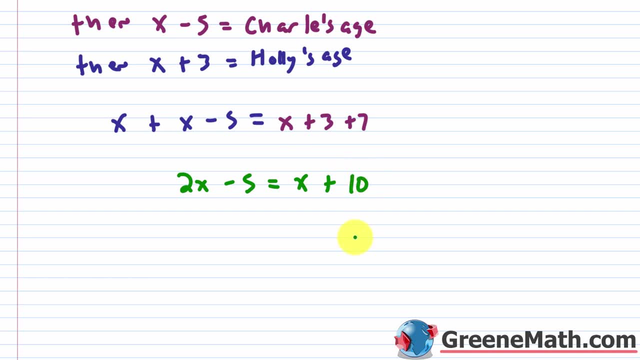 the right. x plus three plus seven is going to give me ten. so what I'm going to do from here is just subtract x away from each side of the equation. I'll also add five to both sides of the equation, and so let's cancel this and cancel this. so what I'm going to have is two x plus three. 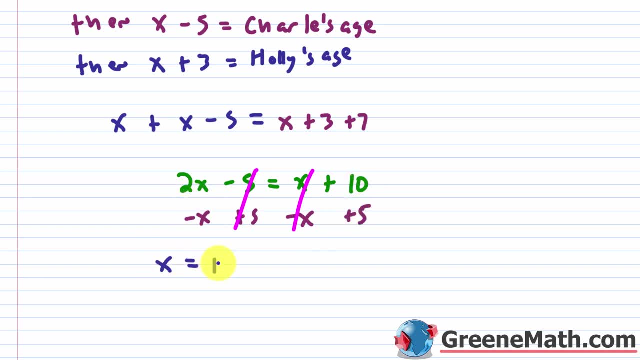 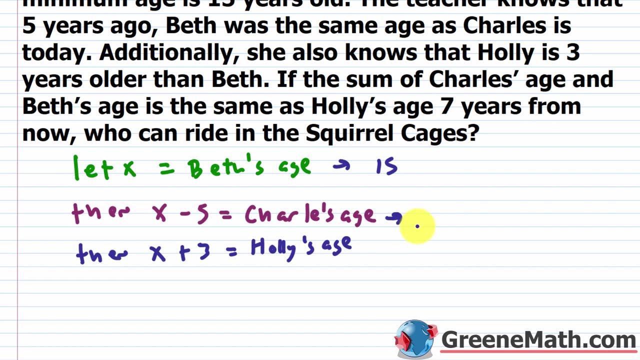 two x minus x is simply x, and this equals ten plus five, is going to give me fifteen. all right, so x is fifteen. so we know that Beth's age is going to be fifteen years old, and then for Charles he's going to be ten years old, because fifteen minus five is ten. and then for Holly, she is going. 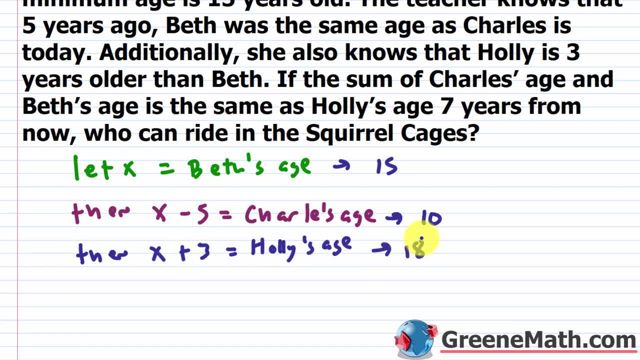 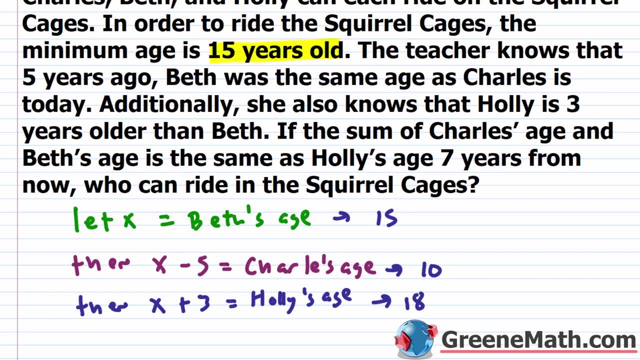 to be fifteen plus three or eighteen years old. so the question actually asks who can ride in the squirrel cages. and again, the minimum age, as we're told here, is fifteen years old. so basically, Beth can't ride, so we'll put a yes for her. Charles cannot ride because he's only ten, so we'll put a. 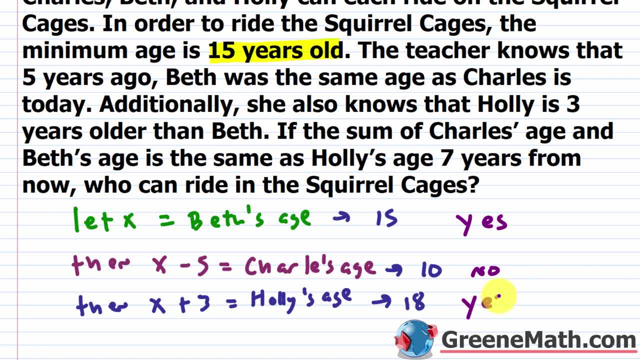 no for him. and then Holly is going to be able to ride because she is 18, so we'll put a yes for her. so going back through this again, we see that the teacher knows that five years ago Beth was the same age as Charles is today. so five years ago Beth would have been 10 and Charles is currently. 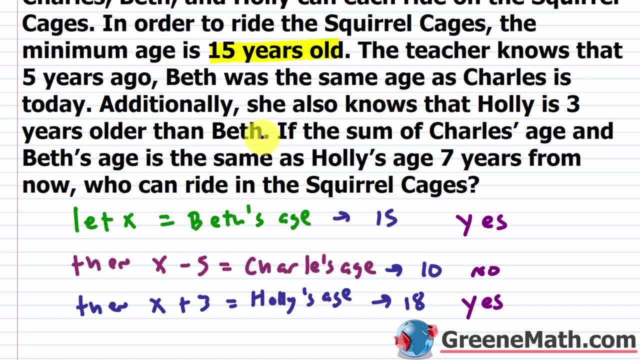 10.. so that checks out. additionally, she knows that Holly is three years older than Beth. well, we know that Holly's 18 and Beth is 15. so that checks out. it says: if the sum of Charles's age and Beth's age, so that would be 15 plus 10, that's going to. 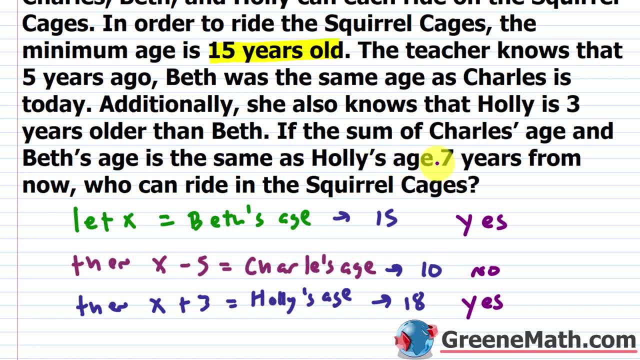 be 25. and then we're saying: is the same as Holly's age seven years from now? well, Holly, seven years from now, is also going to be 25. so that checks out as well. so this is going to be our answer here again: Beth is 15. she's going to be able to ride the squirrel cages. Charles is going to be 10. 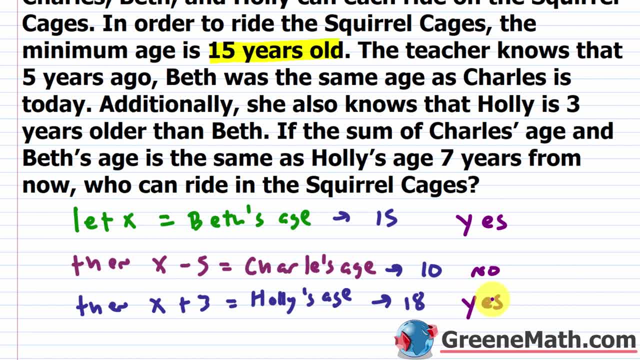 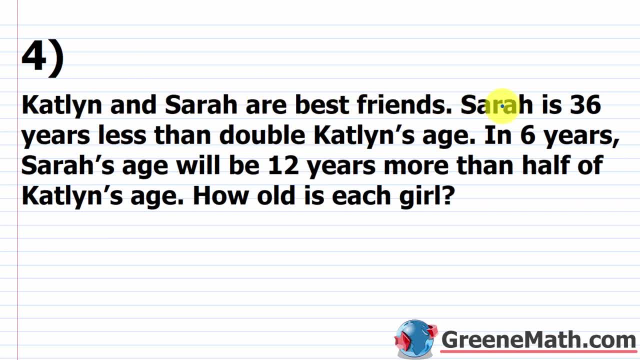 he cannot ride the squirrel cages. and then Holly is going to be 18 and once again, yes, she can ride the squirrel cages. all right, let's look at problem number four. okay, so we have Caitlin and Sarah are best friends. Sarah is 36 years, less than double Caitlin's age. 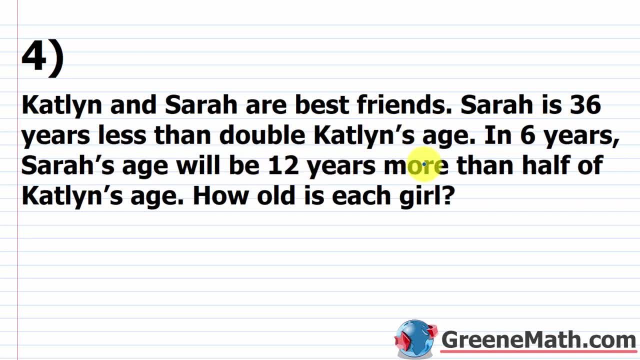 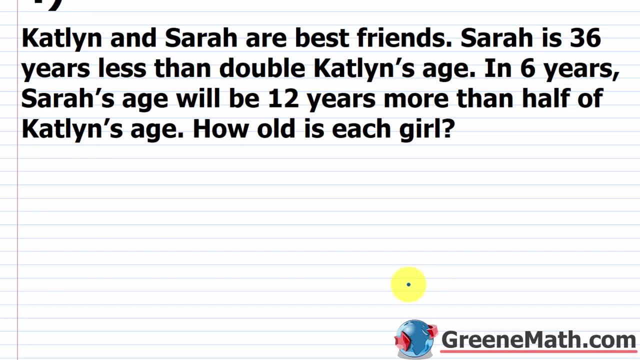 in six years, Sarah's age will be 12 years, more than half of Caitlin's age. How Old Is Each Girl? all right. so, when we think about this type of problem, what you'd want to do here, since we have this statement, Sarah is 36 years, less than double Caitlin's age- what I would do. 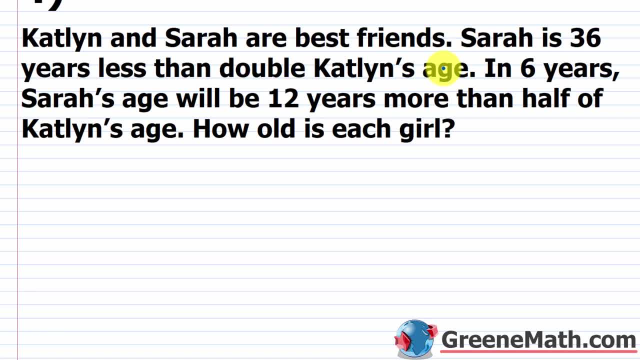 is. I would let X be equal to Caitlin's current age and then model Sarah's current age based on the movie The Hasia 막. he told us it was 25 years. thank God, that is right. we're going to. we can go and look at it more closely. we'll know since then how old is each girl. 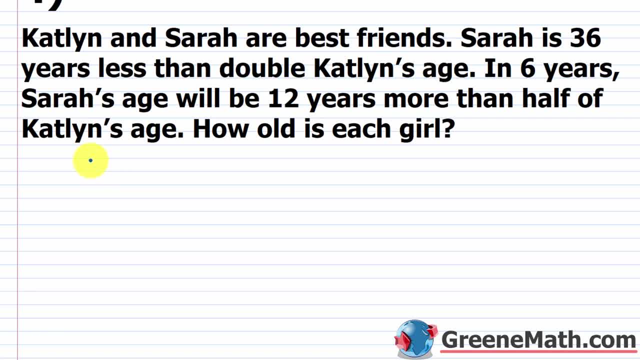 do. I suppose Sarah is 35 years, less than double Caitlin's age. now, over the next year- the question school- I'll ask them: are you coming back age based on that? Okay, So I'm going to start by saying I'm going to let X be equal to. I'm just 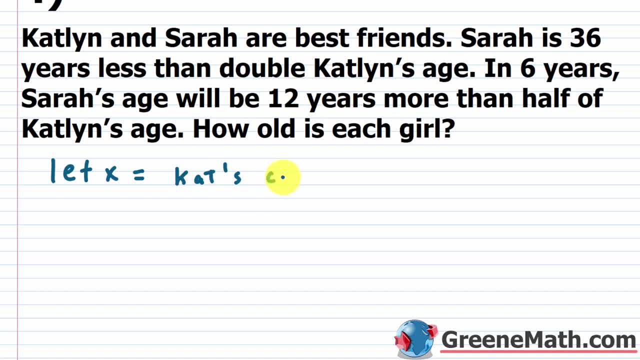 going to put K A, T to abbreviate, So, Caitlin's, you could put current age, I'm just going to put age, Okay. So the next thing is to model Sarah's current age. We have that. it's 36 years less than. 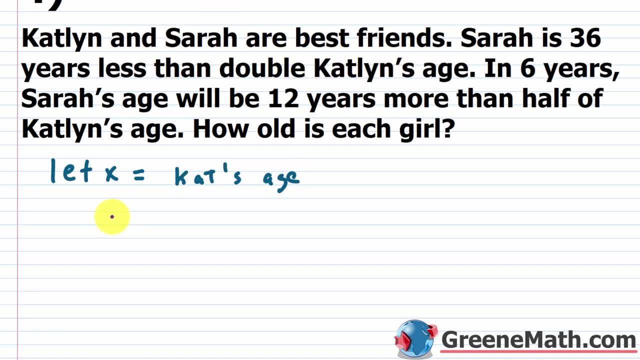 double Caitlin's age. So let me change this up here in the color and we'll put then, if we read this part here where it says double Caitlin's age, well, her age is X, double that as two X, And then we're saying it's 36 years less than that. So I just need to subtract away 36 from. 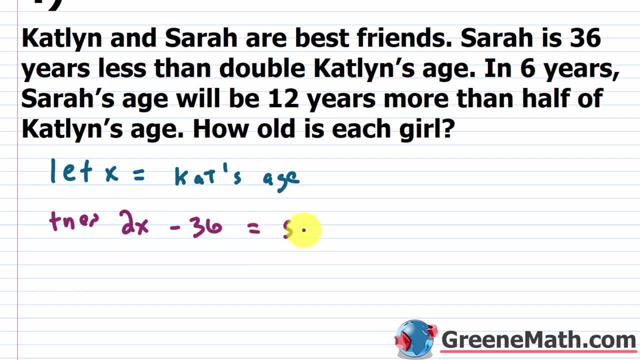 that. Okay, That's all I'm doing. So this would be Sarah. I'm just going to put S A R, So Sarah's current age, I'm just going to put the age there, And then we come to the point here where we need. 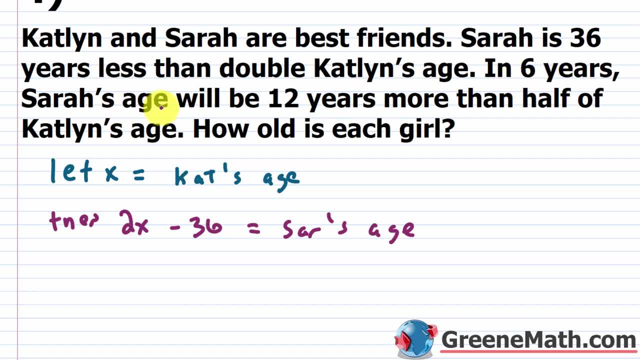 to make an equation. It says: in six years Sarah's age will be 12 years, more than half of Caitlin's age. So this one's a little bit tricky. So I would say I'm going to put, I'm going to put, I'm going. 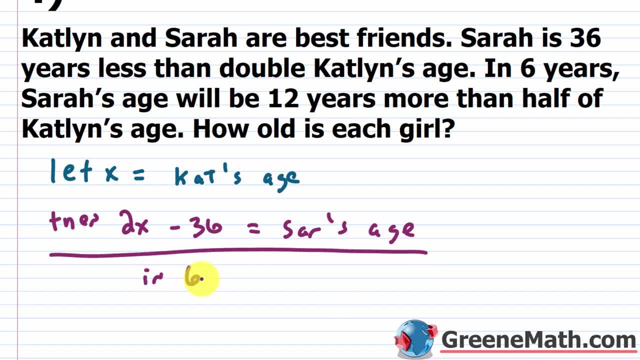 to put a little bar here and say: in six years- And I want to think about how old each girl is going to be then- Well, basically, for Caitlin, she's X years old now. in six years she's going to be X plus six years old. So this is going to be for Caitlin in six years, And then for Sarah. 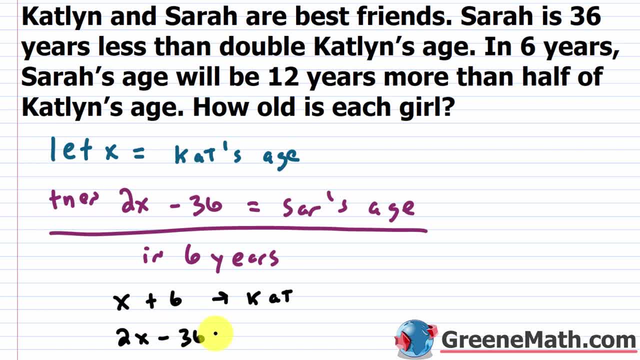 right now she's two X minus 36 years old. Well, in six years I've got to add six to that. So this is going to be for Sarah. So now that we have this modeled in terms of in six years, you can go. 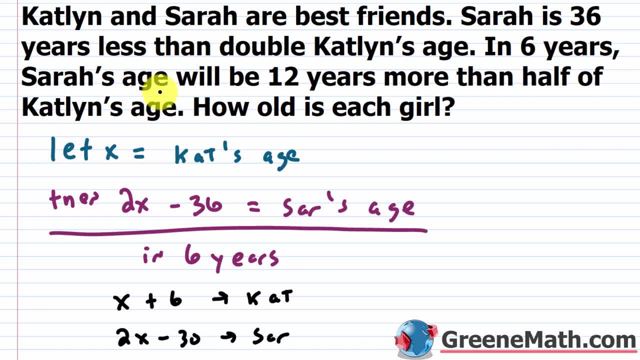 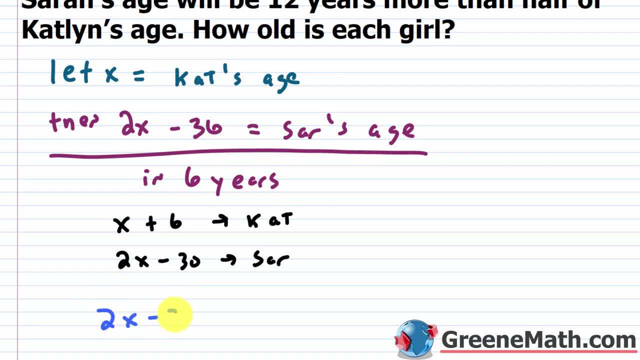 through and make an equation: So in six years, Sarah's age. so Sarah's age, which is given by two X minus 30, I'm just going to write this out: So two X minus 30, then it says we'll be: 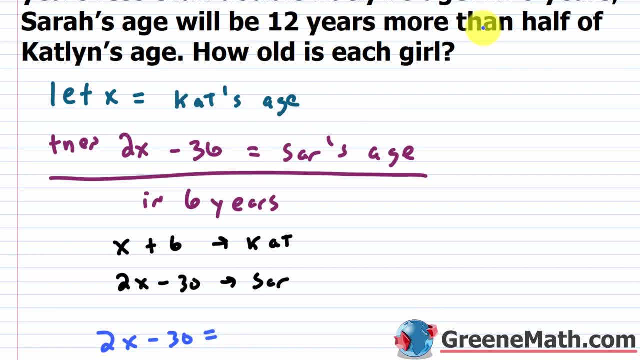 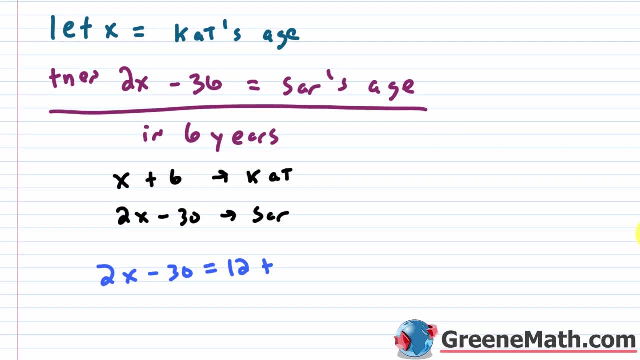 so that just means equals 12 years more than so. 12 years more than that means I'm adding 12 to something half of Caitlin's age. So Caitlin's age again. in six years she's going to be 12 years. 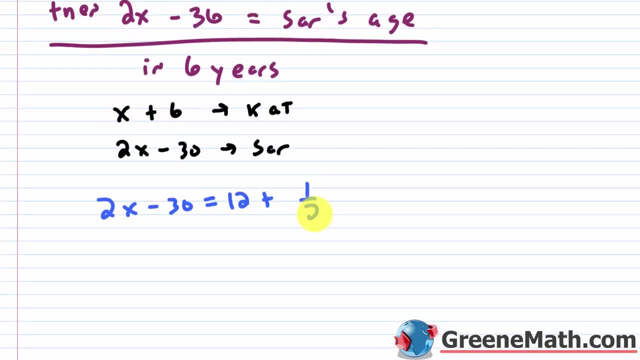 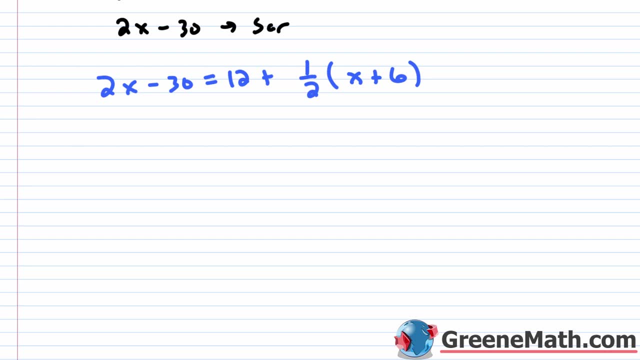 more than six years is represented by X plus six. So if I want half of that, it's half times the quantity X plus six. So this is how we set up our equation here, And so let's go through and just solve this really quickly. You could multiply everything by two just to clear this denominator. 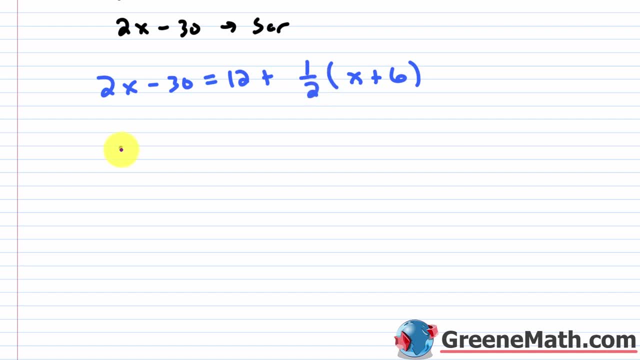 if you want to, But maybe it's a better idea to clean things up first. So let's go to: X minus 30 is equal to 12. And then plus one half times X is a half X, And then plus a half times six is going. 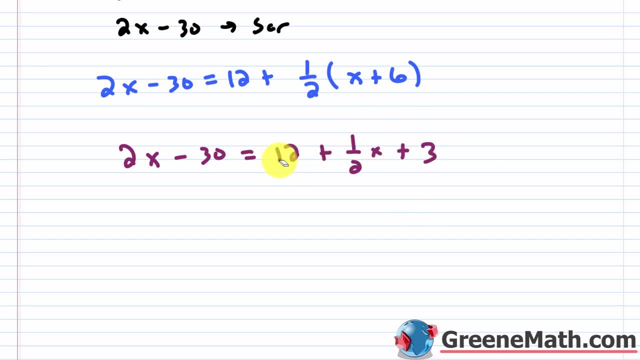 to be three. 12 plus three would be 15.. So let's just arrange that. So let's just arrange that. Let's erase this and put plus 15 over here, like this, And then I can also add 30 to both sides of. 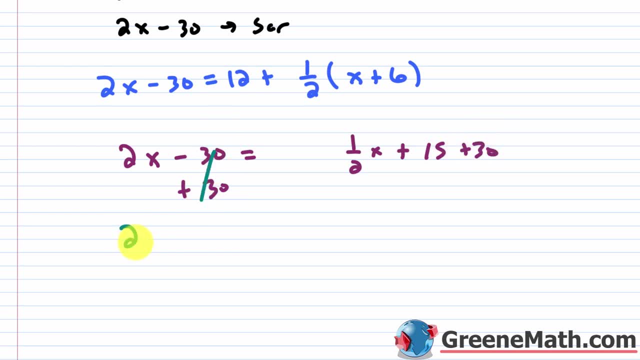 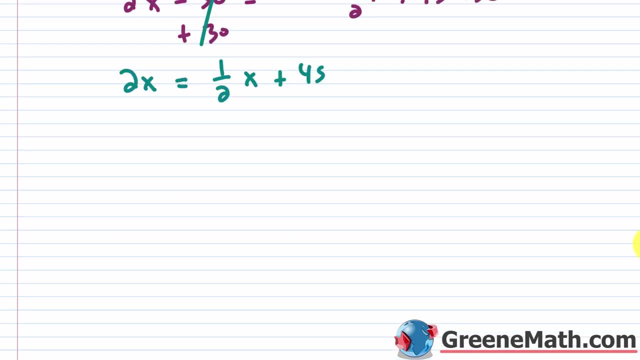 the equation. So let's cancel this And let's say we have two. X is equal to. this would be one half X plus 15 plus 30 is 45. Then from here I just multiply everything by two. now clear the denominator. So this times two would be four X, this times two would just give me one X or just. 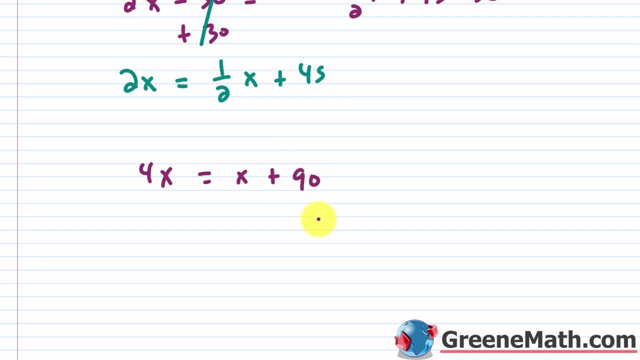 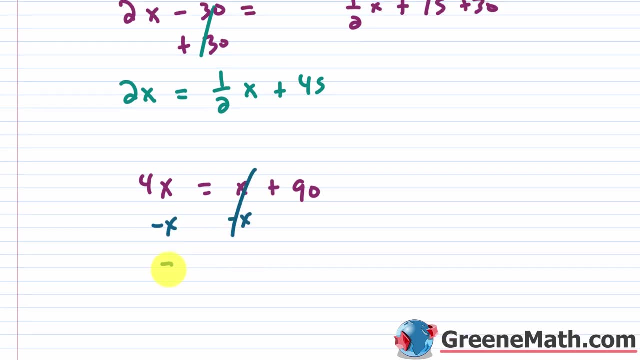 X And then plus this times two would give me 90. So basically from here, really easy to solve this: I would subtract X away from each side of the equation. So this is going to cancel. we're going to have three. X is equal to 90, divide both sides of the. 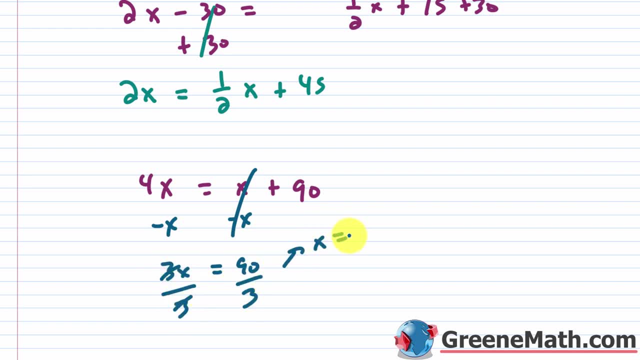 equation by three. this cancels and we're going to get that. X is equal to 90, over three is going to be 30. Okay, so, coming back up here, we always want to check things And I want to put that she's. 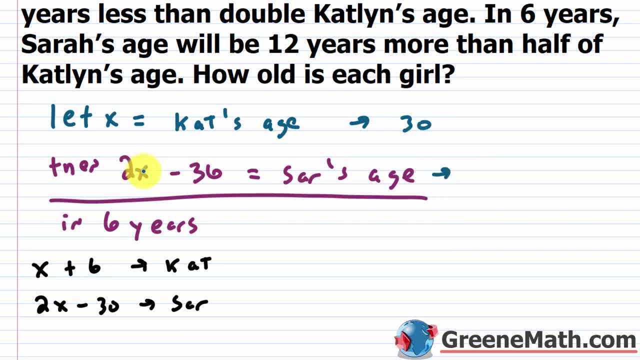 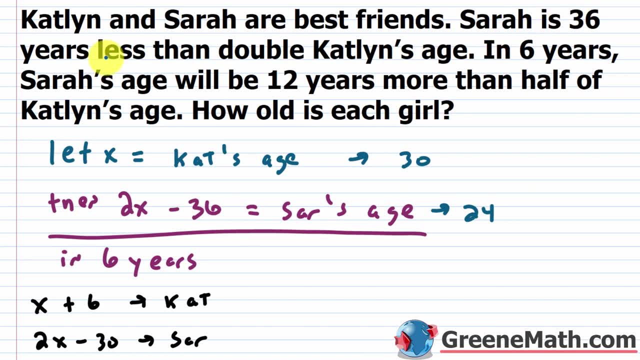 going to be 30 for Caitlin and she's going to be two times 30 is 60, 60 minus 36 is going to be 24.. So Caitlin is 30 and Sarah is 24.. So it says that Sarah is 36 years. 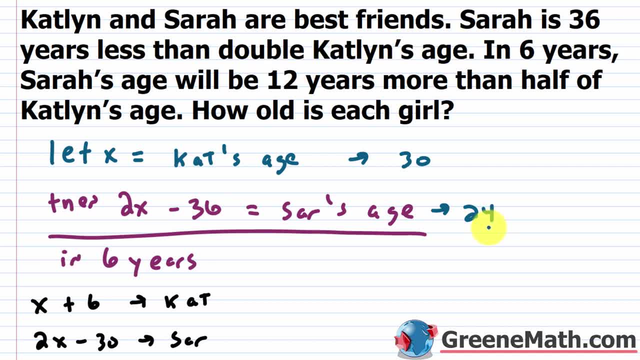 less than double Caitlin's age. Does this check out? If I double Caitlin's age I'd get 60. If I take 36 away from that I get 24.. So that part checks out. Then we have in six years and we're. 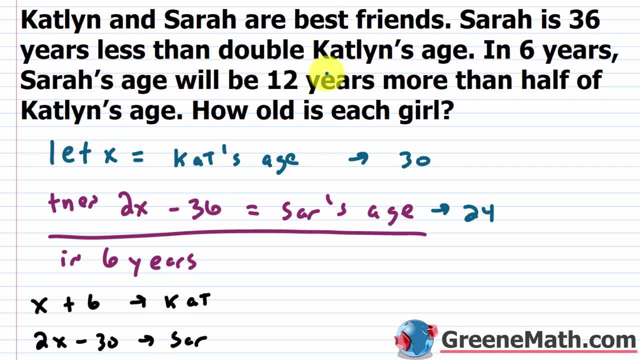 going to need to use this part here. Sarah's age will be 12 years, more than half of Caitlin's age. Well, in six years Caitlin's going to be 36.. And Sarah is going to be 30. Well, half of Caitlin's. 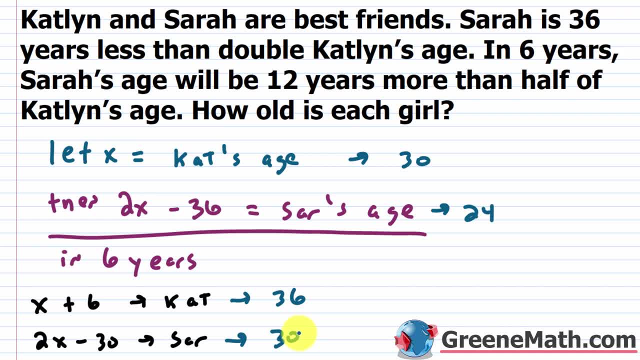 age is going to be 18 at that point And we can say that 30 is 12 years more than 18.. So that part checks out as well. So we have the correct solution here. We'll say Caitlin is 30 years old and Sarah is 24 years old. Alright, let's take a look at problem number. 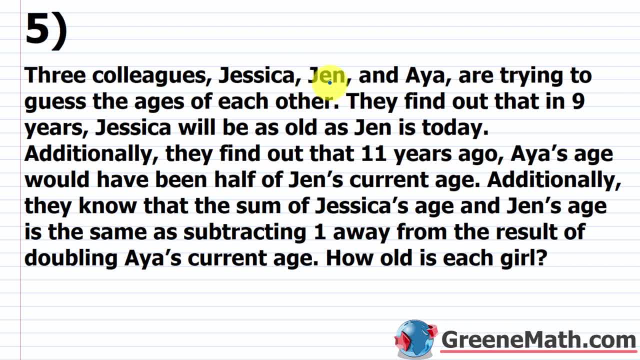 five. So we have three colleagues: Jessica, Jen and Aya are trying to guess the ages of each other. They find out that in nine years, Jessica will be as old as Jen is today. Additionally, they find out that 11 years ago, Aya's age would have been half of Jen's current age. 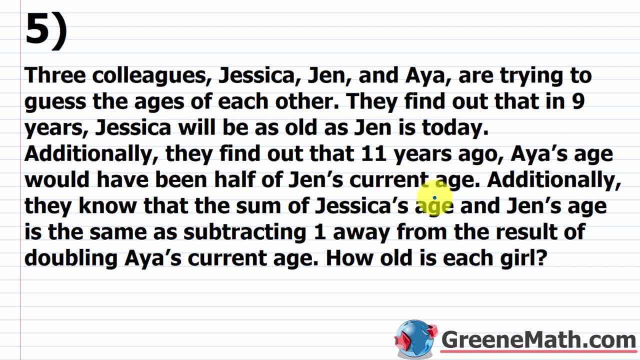 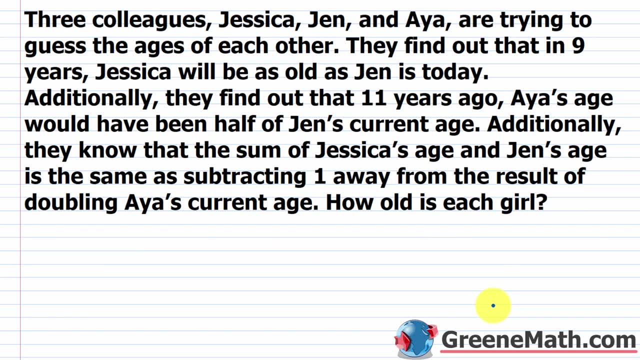 Additionally, they know that the sum of Jessica's age and Jen's age is the same as subtracting one away from the result of doubling Aya's current age. How old is each girl? And let's first again think about who is involved in each comparison. Well, if I come back up here, 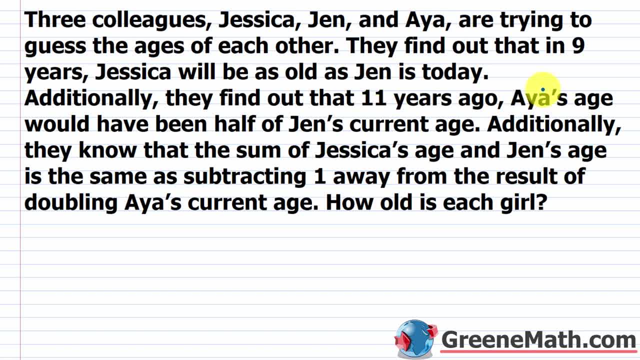 you see that you have Jessica and Jen, And then here you have Aya and Jen. Okay, so I'm going to use Jen- she's involved in each comparison- And I'm just going to let x be equal to Jen's age, So Jen's age like this. Again, if you want to do it a different way, that's up to you. 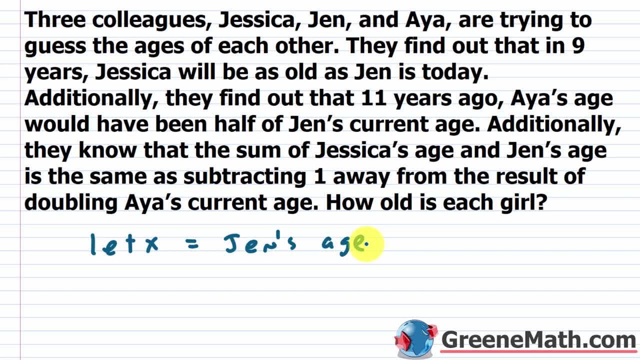 you'll get the same answer. So then, the other thing I want to do is I now want to go back through here And I want to see: will they find out that in nine years, Jessica will be as old as Jen is today? Well, that means that basically, Jessica is nine years younger than Jen. So I'm 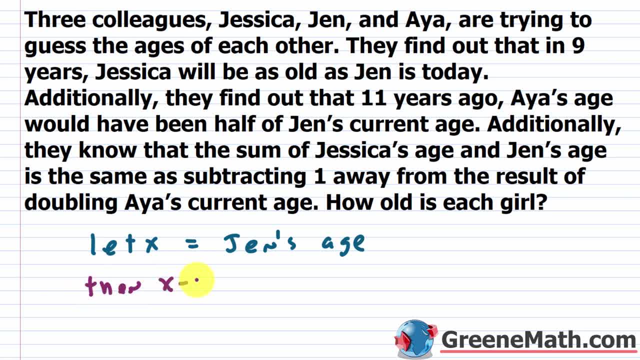 just going to say: then we'll have: x minus nine is equal to Jessica's age. So Jessica's age- and maybe I'll make these ease a little bit better here- So let's fix that, Okay. then, lastly, we need to think about Aya. So it says: additionally, they find out that 11 years ago, 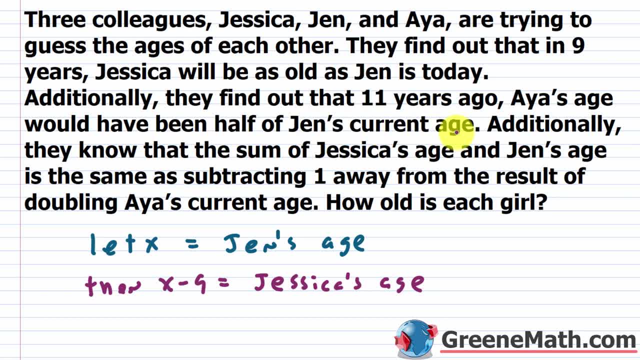 Aya's age would have been half of Jen's current age. Now, I know these are tricky, but just start out with half of Jen's current age. What is that? Well, Jen is currently x years old, So half of that is one half x. Let me do this in a different color So we can keep track of things. So I'm 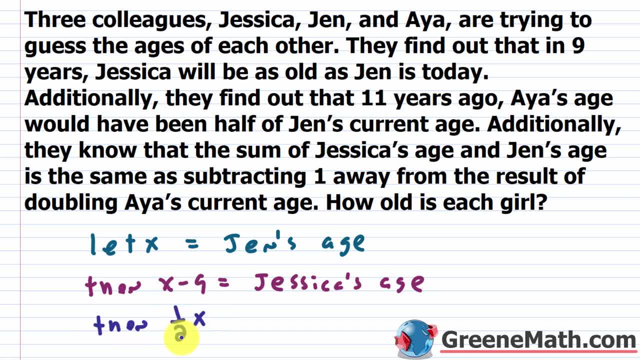 going to put then here and then I'm going to put one half x, and that just represents half of Jen's current age. Now, this is not the current age for Aya, because it says this would have been 11 years ago, right? So to get to the current age of her, or to get to the current time period that we're in 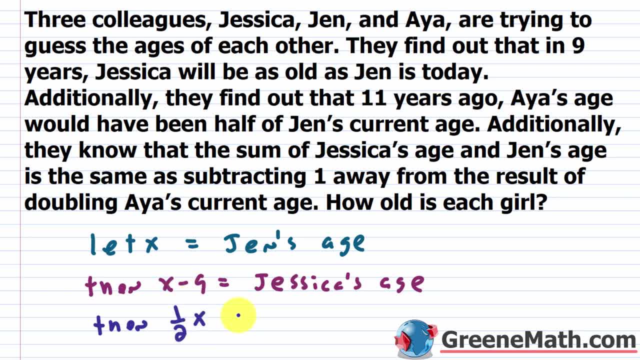 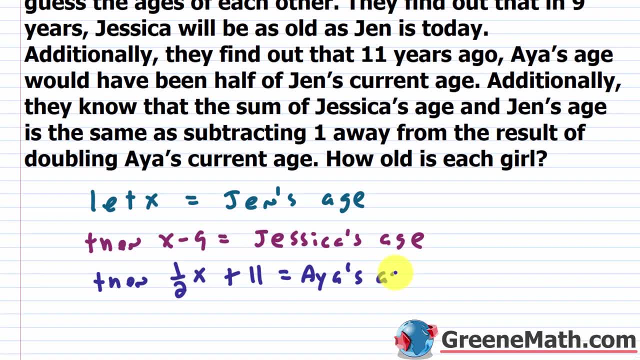 we need to add 11 to this result, right? Because this is 11 years ago. So I'm going to add 11 to this, And this is going to give me Aya's current age, right? So Aya's age. Okay, so let's go through. 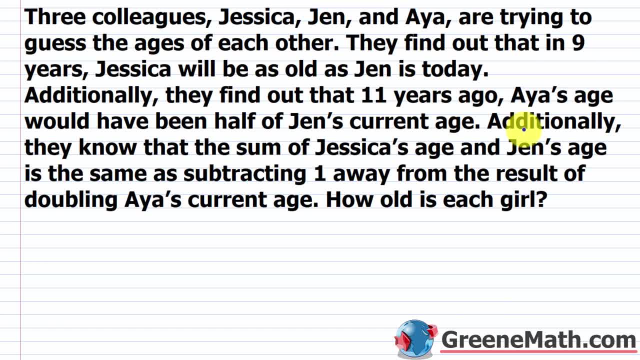 here and see if we can get an equation going- And we're going to focus on this last part right here- where it says: additionally, they know that the sum of Jessica's age and Jen's age is the same as. So let's go back. 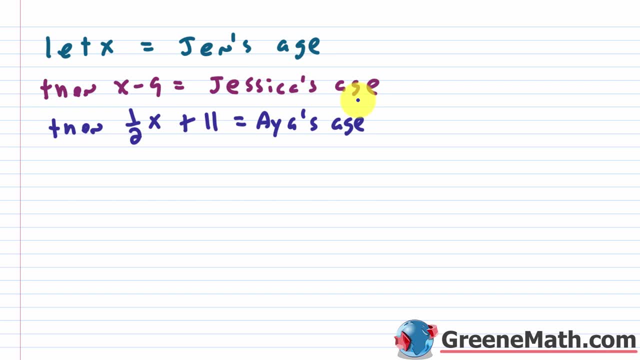 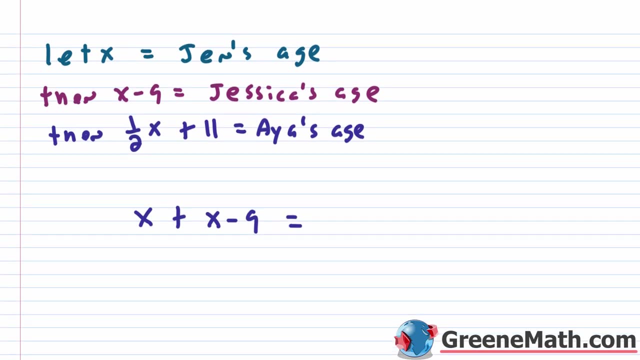 So you have Jen's age here and Jessica's age here. We're going to sum them, So we're going to have x plus x minus nine and we're going to say equals. right Is the same as means equals. Let's go back. 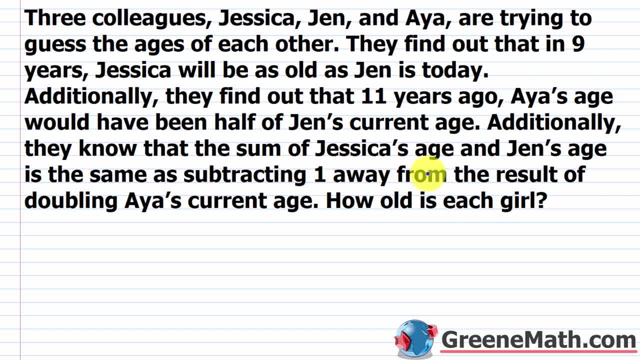 And then, just coming back here, it says as subtracting one away from the result of doubling Aya's current age. So I want to double Aya's current age. So I'm going to double Aya's current age and then I want to subtract away one. So over here on the right, I want to double Aya's. 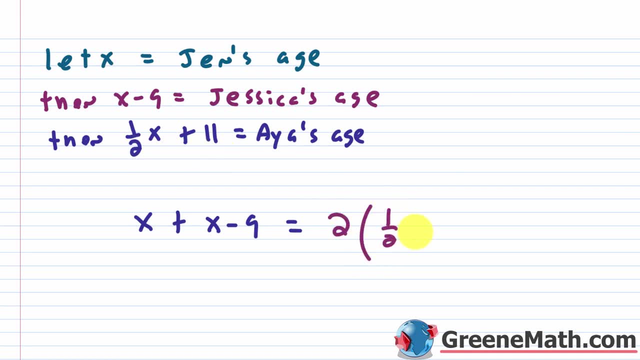 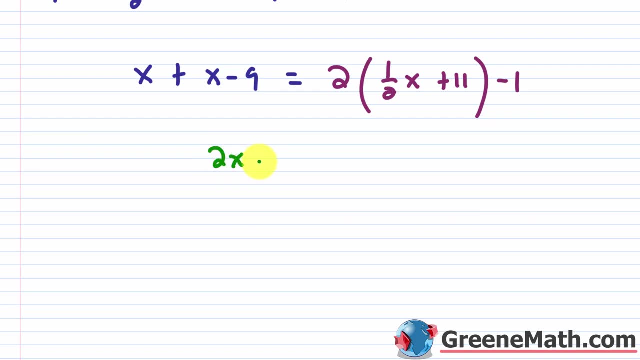 current age. So that is two times the quantity one half x plus 11.. And then I just want to subtract away one. Okay, so this is our equation. So we know that x plus x is two. x and then minus nine is equals. two times a half is just one. So this is just x, And then plus two times 11 is 22.. 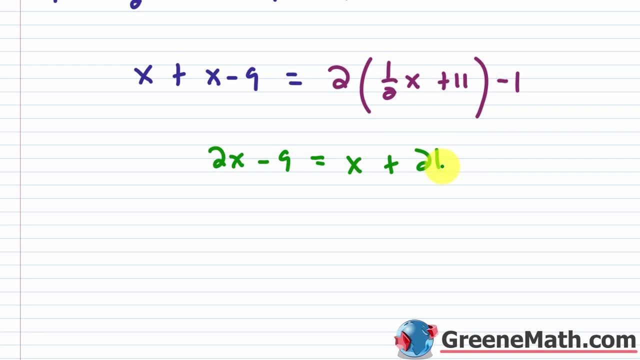 You're subtracting away one. let's just write this as 21 here, And what I'm going to do from here is just add nine to both sides of the equation. Subtract x away from each side of the equation. This is a real easy one to solve. this cancels this. 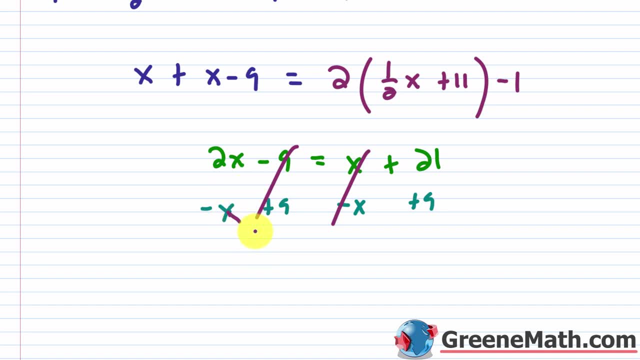 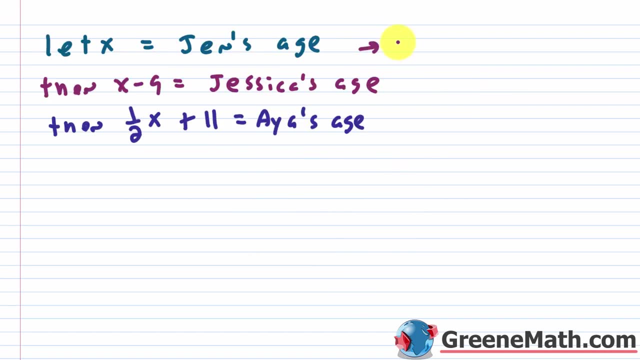 cancels two x minus x. Let me make this x better. So two x minus x is going to be x. This equals 21 plus nine is going to be 30. So 30 is going to be the age for Jen. So she's going to be 30.. Jessica. 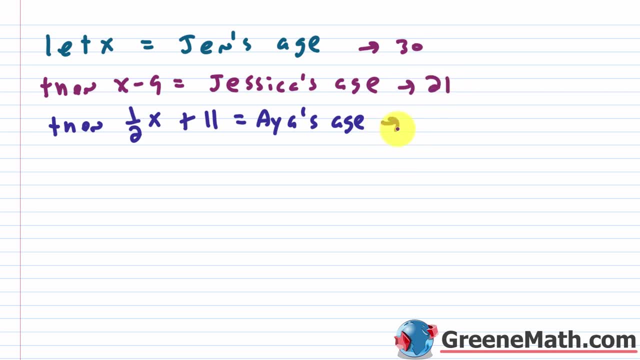 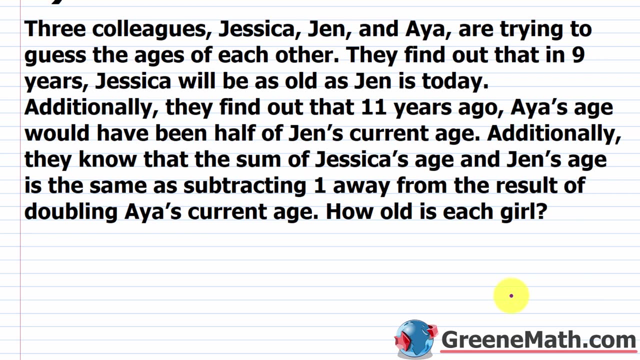 is going to be 30 minus nine or 21.. And then Aya is going to be 30 times a half, which is 15 plus 11, which is going to be 26.. And because that stuff's on the other screen, we need a way to. 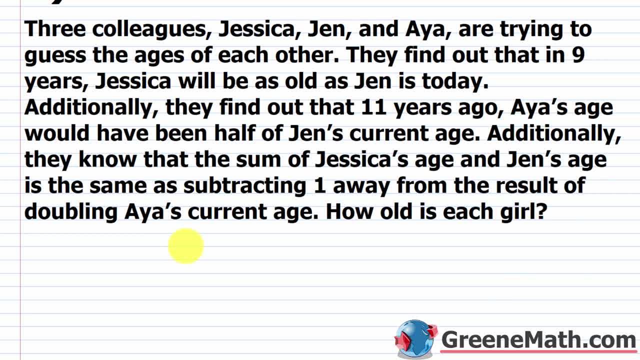 reference things when we check it. Let's just write something simple. I'm not going to make a sentence, I'm just going to put that: Jen- and let's make this E better here So it's legible- So Jen is going to be 30. And let's put that. 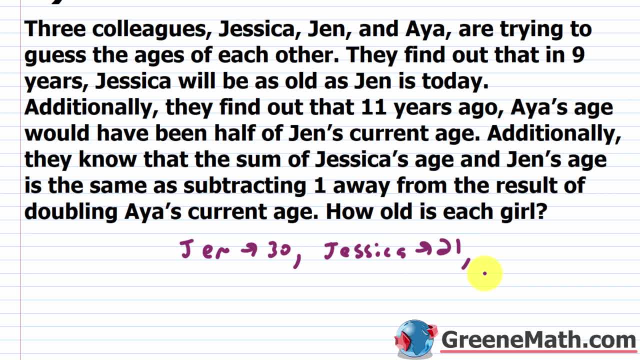 Jessica. So Jessica is 21.. And then, Aya, we know she is going to be 26.. Okay, so let's just read back through, make sure everything makes sense. So they find out that in nine years, Jessica will be as old as Jen is today. Well, right now Jen is 30. In nine years, Jessica will be 21 plus nine. 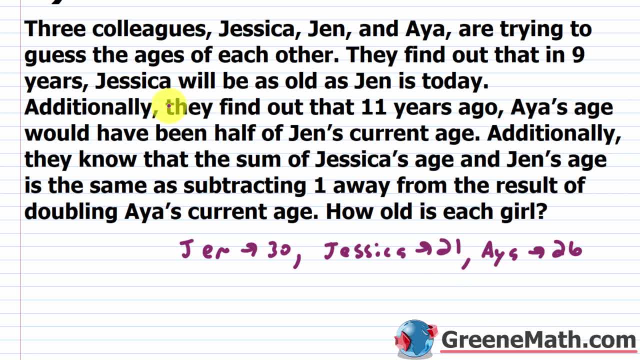 or 30. So that works out. Then, when we think about the other guy we have, they find out that 11 years ago Aya's age would have been half of Jen's current age. Well, 11 years ago Aya would have been 15. And that is. 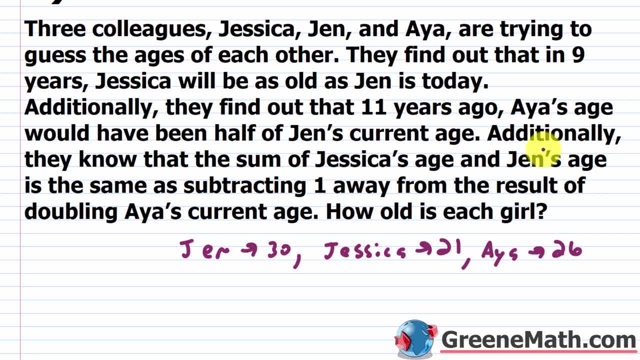 half of Jen's current age, which is 30. So that checks out. Then we have additionally, they know, the sum of Jessica's age and Jen's age. So 30 plus 21 is 51 is the same as subtracting one away. 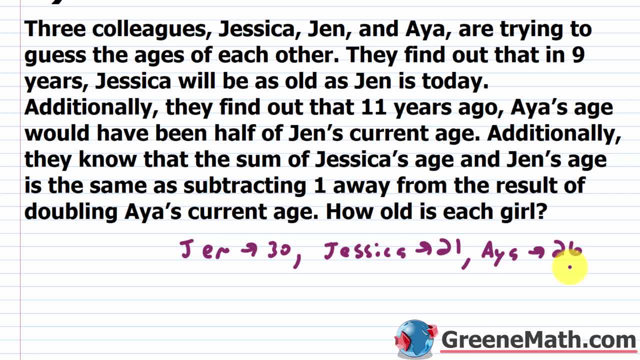 from the result of doubling Aya's current age. If I double 26,, I get 52. Take one away, you get 51. So everything checks out here. So Jen is 30. Jessica is 21. And Aya is 26..